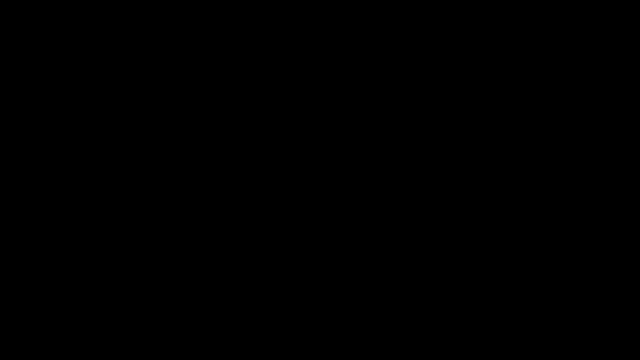 In this video we're going to focus on naming carboxylic acids, So let's start with some common examples. Here we have a one carbon carboxylic acid molecule, and so the common name for this is formic acid. The IUPAC name for it is called. 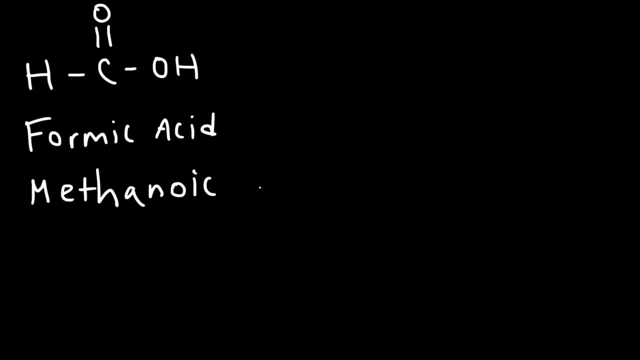 methanoic acid, since we have one carbon in this molecule. In this example, we have two carbons. The common name for this particular carboxylic acid, as you no doubt heard before, is acetic acid and the IUPAC name ethyl. 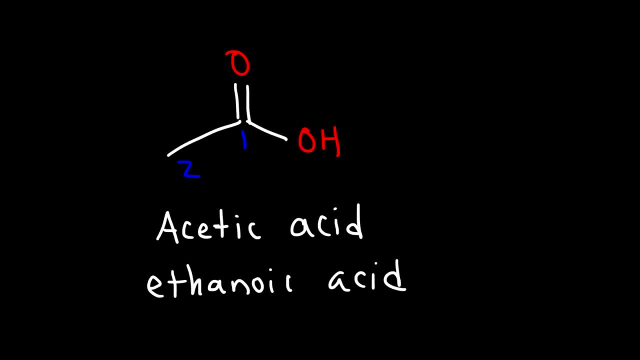 ethanoic acid. Next up, we have a four carbon carboxylic acid, and it looks like this. So the common name for this is butyric acid and the IUPAC name is butanoic acid, Since we have a total of 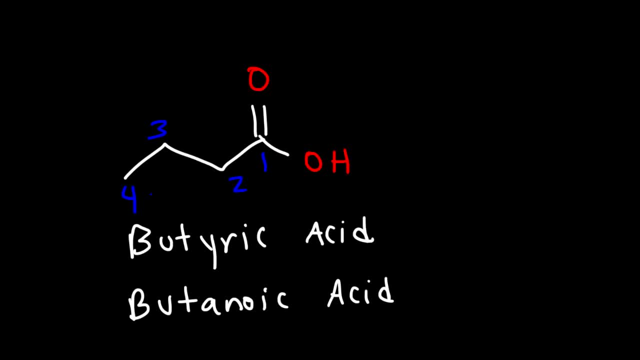 four carbon atoms in this molecule. So here is another example. Go ahead and write the common name and also the IUPAC name for this particular molecule based on the last example. So let's start with the common name. We know that four carbon carboxylic acid is called butyric. 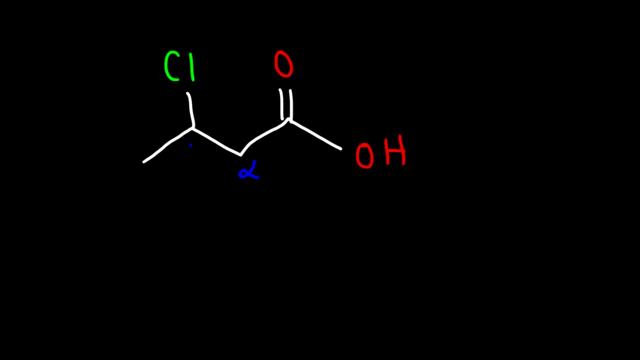 acid. This is the alpha carbon. the second carbon is the beta carbon and this is the gamma carbon. so this is called beta chloro butyric acid. now for the iupac name. this is going to be carbon 1234, so it's also called 3-chloro-butanoic acid. go ahead and try. 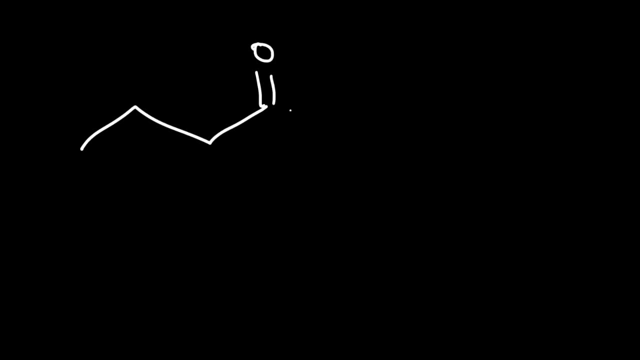 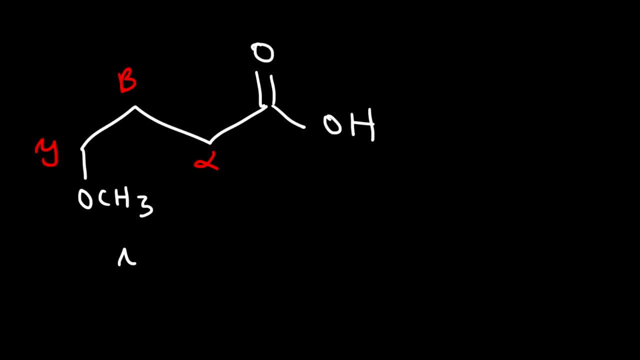 beta carbon. this is beta and this is gamma. so the common name: this is going to be called a gamma methoxy butyric acid. now for the iupac name: this is carbon 1234, so this is going to be called 4-methoxy butanoic. 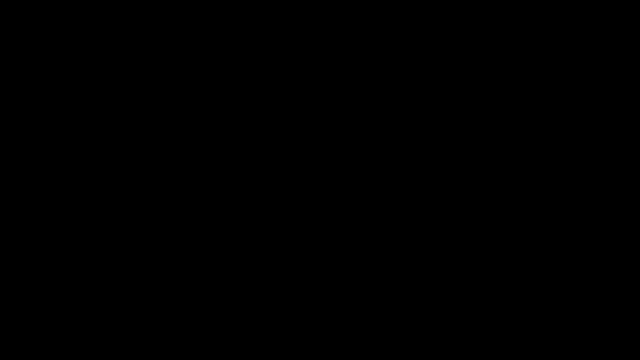 acid. for our next example, we're going to have a six carbon carboxylic acid molecule with an NH2 group attached to it. so what is the iupac name for this molecule? as always, we're going to start counting from the carboxylic acid, so the 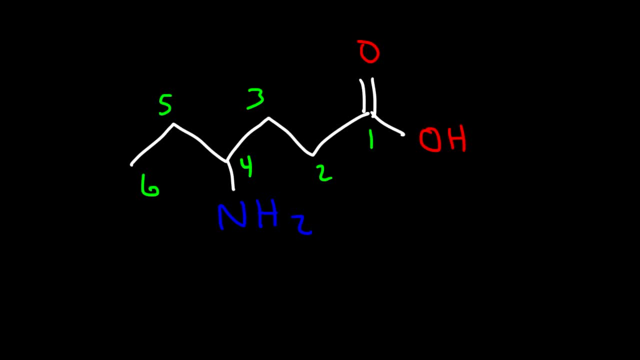 NH2 group is on carbon 4 as a substituent. the NH2 group is called amino, so this is going to be for amino and since we have six carbons in the parent chain, hexane. but with the carboxylic acid functional group, it's going to be called hexanoic acid, and so 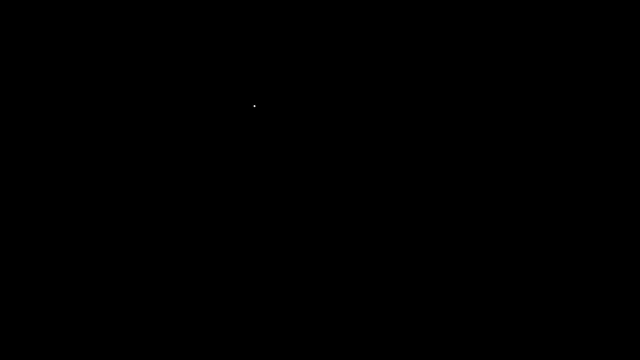 that's the name for amino hexanoic acid. now for our next example. we're going to have this molecule, so we're going to have a ketone functional group and the mean and also an ether. go ahead and name the molecule so carbon. one has to be the carbon with the. 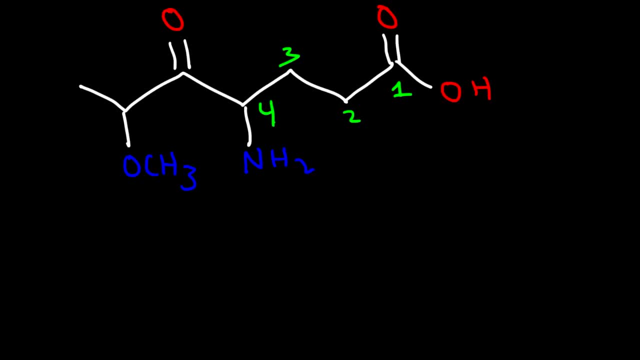 carboxylic acid, it has the highest priority. the amino group is on carbon 4, we have a ketone on carbon 5 and a methoxy group on carbon 6. so how can we put this together? well, we need to put it in alphabetical order, so the amino group comes first. so 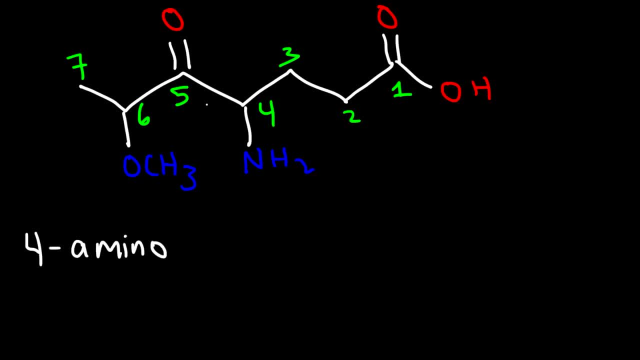 it's going to be for amino. and then here we have a methoxy group compared to the ketone which, as a substituent, is called oxo. so M comes before O in the alphabet. so this is going to be for amino 6, methoxy. and then 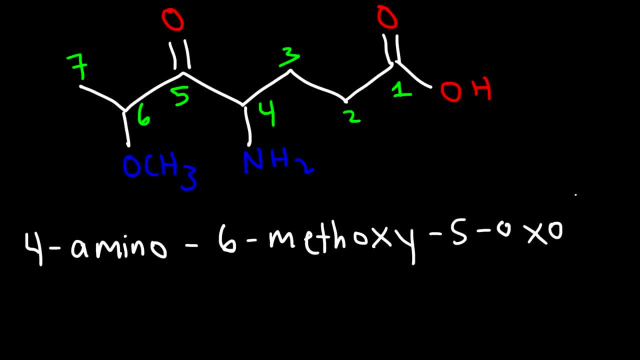 5 oxo and finally heptanoic acid, and so that's how we can name this molecule. so 4 amino 6 methoxy, 5 oxo, heptanoic acid. next up we have this molecule. so what do you think the name for this molecule is? 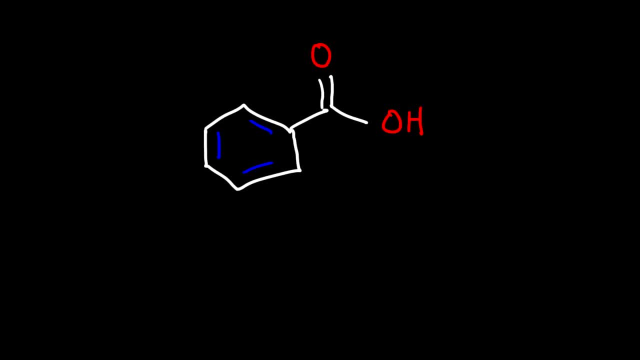 called. so we have a benzene ring and a carboxylic acid. this is known as benzoic acid. now what if we didn't have a benzene ring? let's say, if we have a cyclohexane ring instead, with the carboxylic acid attached to it. so how can we name this? 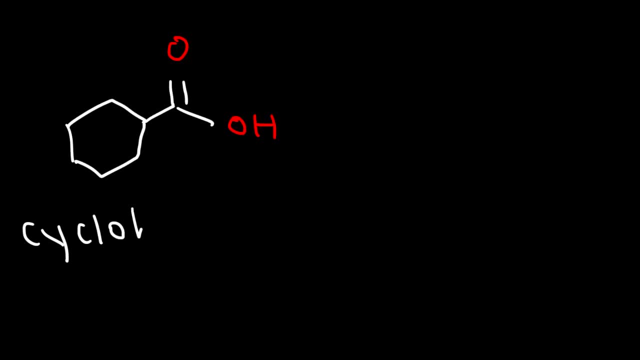 this is called simply cyclohexane carboxylic acid. likewise, let's say, if we have a cyclopentane ring with the carboxylic acid functional group, this is going to be called cyclopentane carboxylic acid. now go ahead and try. 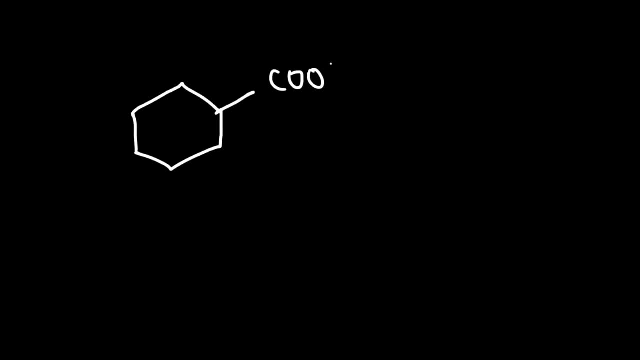 this one? what is the IUPAC name for this molecule? so we have a cyclopentane ring, a carboxylic acid, so those two combined combine is cyclohexane carboxylic acid. but now we have a methyl group attached to it. this is automatically carbon one due to the carboxylic acid, and so this: 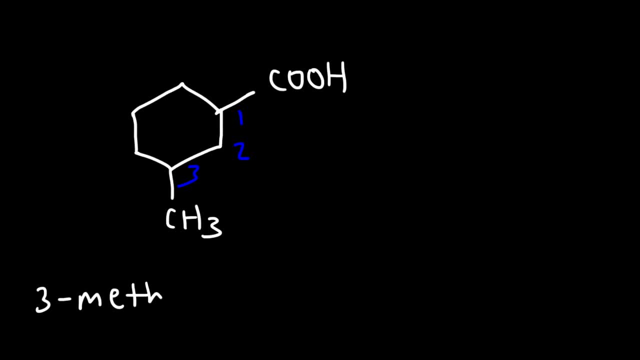 is going to be called 3-methyl cyclohexane carboxylic acid, and so that's how we can name that molecule. now let's try another example. so let's say we have a cyclohexane ring attached to a chain that contains the carboxylic. 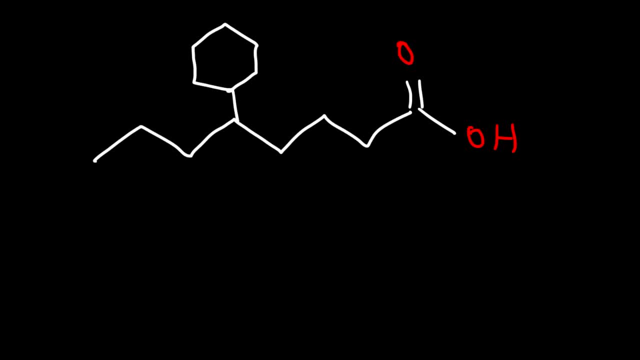 acid. what's the name for this molecule? so now this is going to be a substituent, so it's going to be called cyclohexyl with a YL instead of cyclohexane, and so that's how we can name that molecule. now let's try another example. 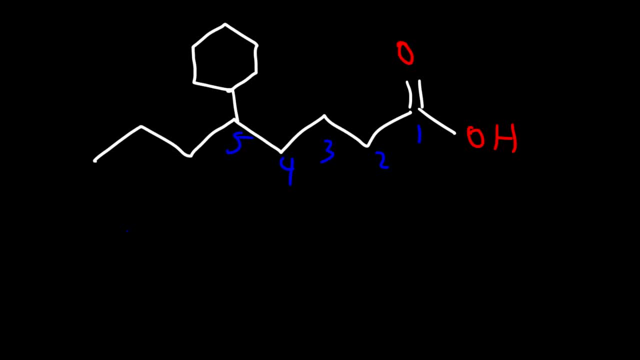 and so that substituent is going to be on carbon 5 and we have an, a carbon chain. so instead of saying octane is going to be octanoic acid. so, to put it all together, this is 5 cyclohexyl and then octanoic acid. 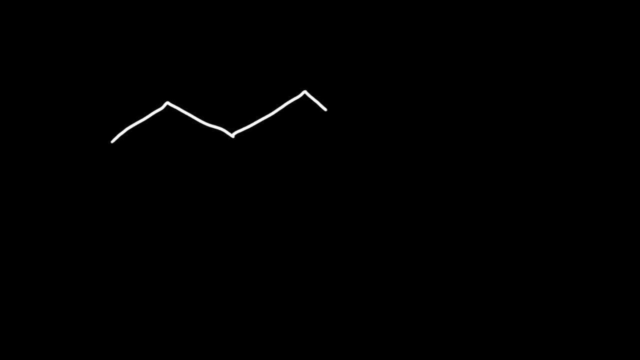 now let's move on to our next example. so this time we're going to have an alkene functional group with a carboxylic acid. so go ahead and NATO. so this is going to be carbon one, two, three, four, five, six. so we have the alkene on carbon three and the carboxylic acid on carbon one. so this is. 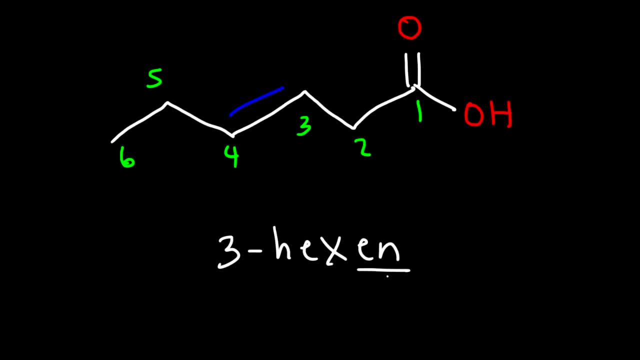 going to be three, two, three, four, five, six. so that's is the right answer. you need hexene ene for the alkene and then oic for the carboxylic acid, So 3-hexene-oic acid. 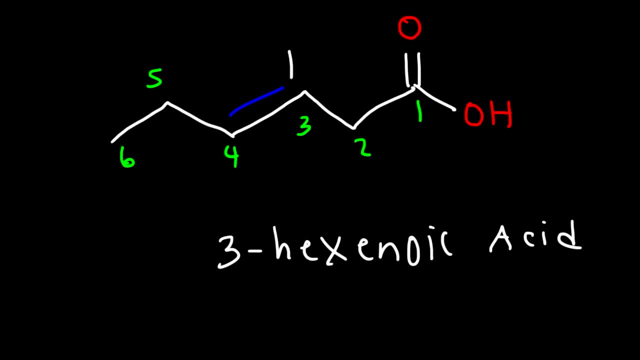 Now the hydrogen atoms notice that they're opposite to each other, And so we have the trans isomer as opposed to the cis isomer. So this is trans-3-hexenoic acid. Now, sometimes you'll be given a molecule with two carboxylic acids. 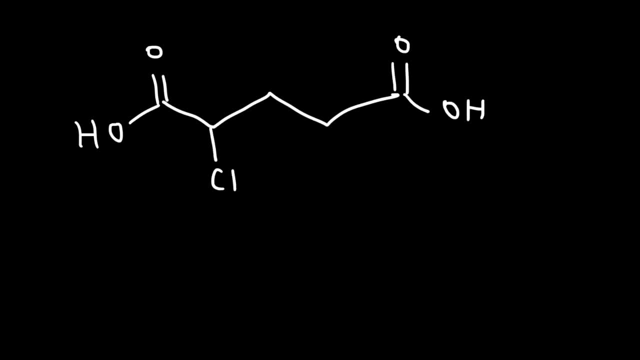 And so this is going to be called a dioic acid. Now we need to number it from left to right, because the methyl group will be on carbon-2 as opposed to carbon-4. And so, to put this together, this is going to be 2-methyl. 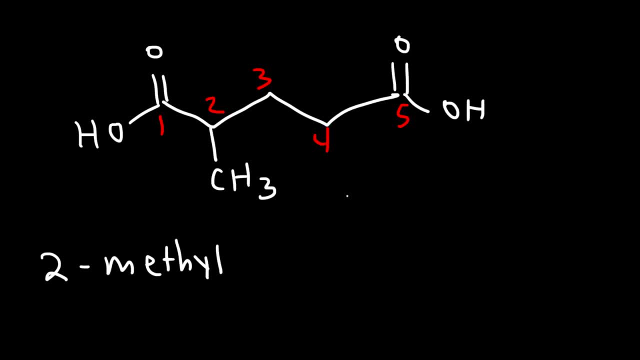 And then we have a 5-carboxylic acid Carbon chain, so pentane, 2-methylpentane and then dioic acid. So here's another one that we could try. Feel free to pause the video and work on this example. 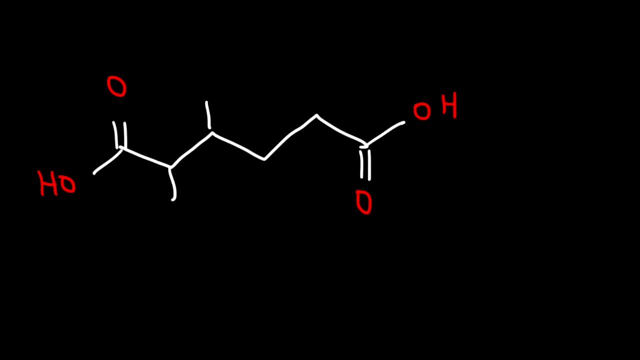 So this time we're going to have a bromine atom attached And also an OH group. Go ahead and name the molecule. So, since the substituents are on the left side, we're going to make this one carbon-1.. 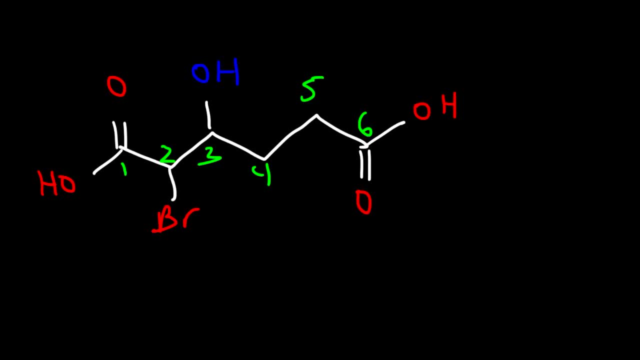 So you need to number it in such a way that the substituents have the lower numbers, And now we need to put it in alphabetical order, So bromo will come before the hydroxy group. So this is going to be 2-bromo. 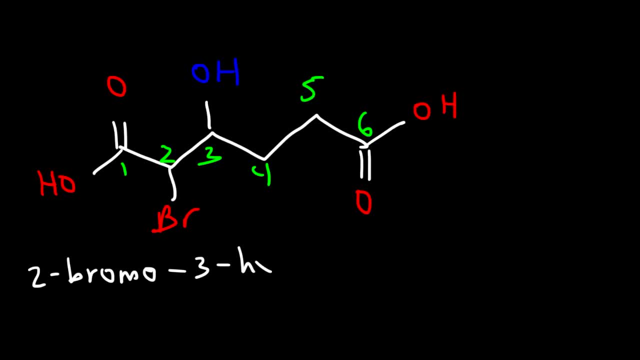 And then 3-hydroxy. Now we have a 6-carbon chain, So this is going to be hexane And then dioic acid. So that's how we can name this molecule: 2-bromo, 3-hydroxy, hexane, dioic acid. 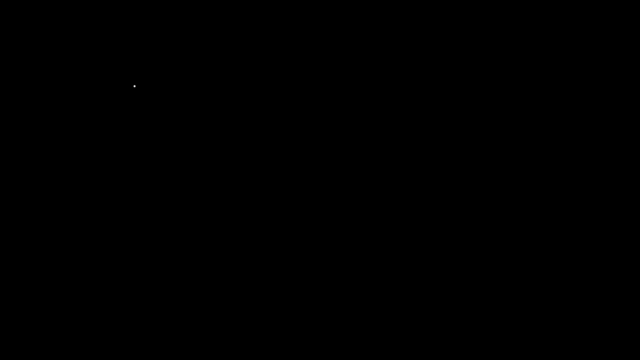 Now let's go over some common names. Let's go over some common names of dioic acids. So if you have a 2-carbon dioic acid, the common name is oxalic acid. Now for a 3-carbon dioic acid, the common name is malonic acid. 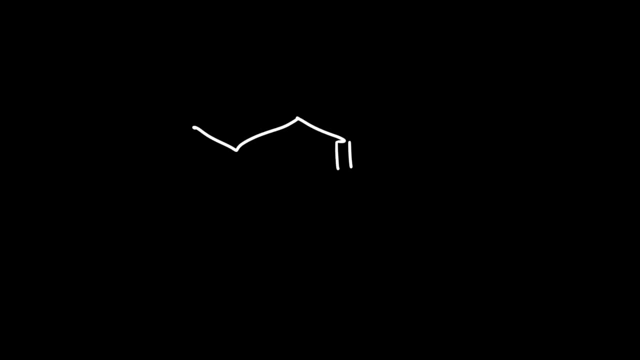 So 5-carbon are hypochloric acid. And how about a 4-carbon dioic acid? the common name for this is succinic acid, And here are some other examples. So here we have a 5-carbon dioic acid.